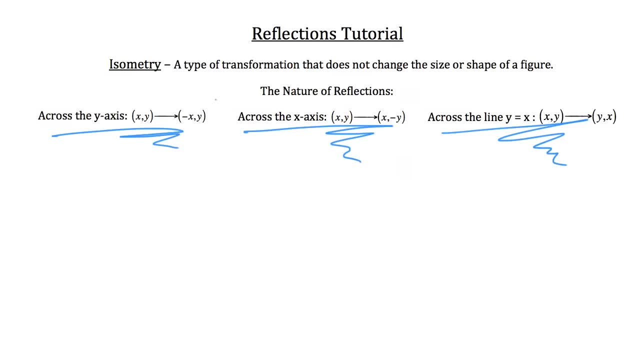 So it's always just the opposite of what the y was originally. Lastly, when looking at a reflection across the line, y is equal to x. all we have to do in this case is take what the original coordinate point was for one of the coordinates in that figure. 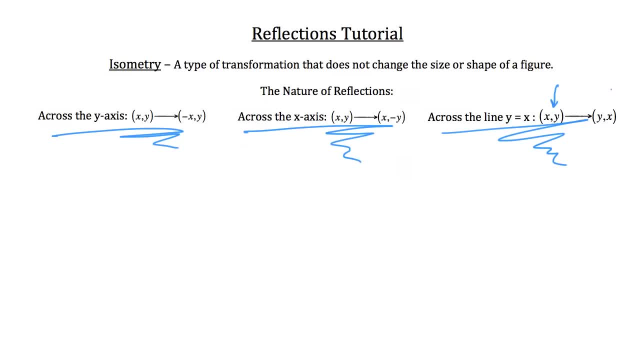 and switch the x and y coordinates of that coordinate point. So now the y comes first, The y is the new x and the x is now the y. And I'm going to show you an example of each of these types of reflections so you really understand the nature of each reflection. 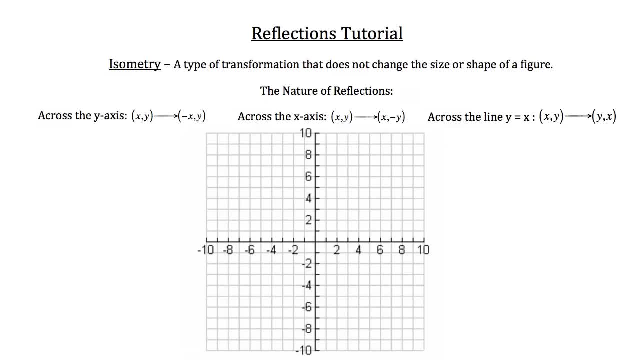 Let's go ahead and put a graph in here and we're going to drop a figure into our graph. I'm going to drop in triangle AB Over here on the left. I'm going to indicate the points, the coordinate points, for each of those letters: A, B and C. 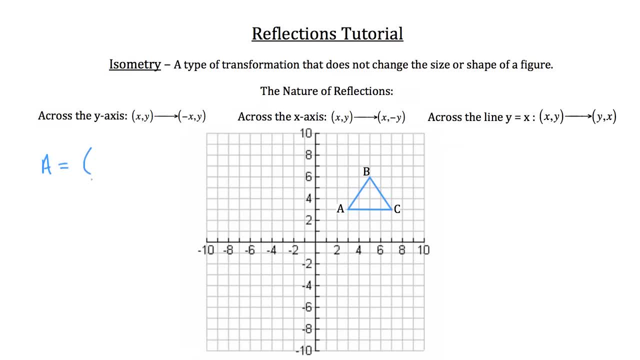 So A occurs at coordinate point And B occurs at coordinate point. Lastly, C occurs at the coordinate point. Alright, so now we have the coordinate points of each of the original points that makes up triangle ABC. Now, first we want to reflect that triangle ABC across the y-axis. 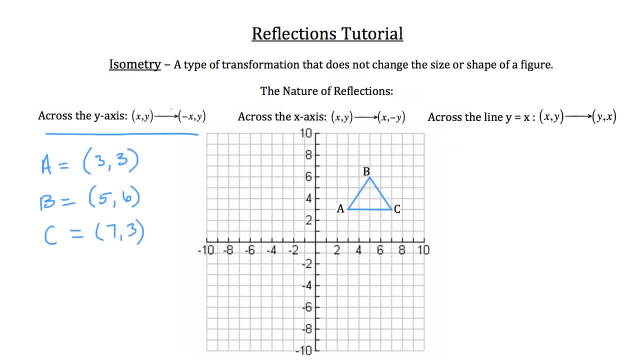 Now, in order to reflect it across the y-axis, remember, I've got to just take what our original point was and add a negative in front of the x, So I'm going to go ahead and write that point here For A. the new point is going to be: 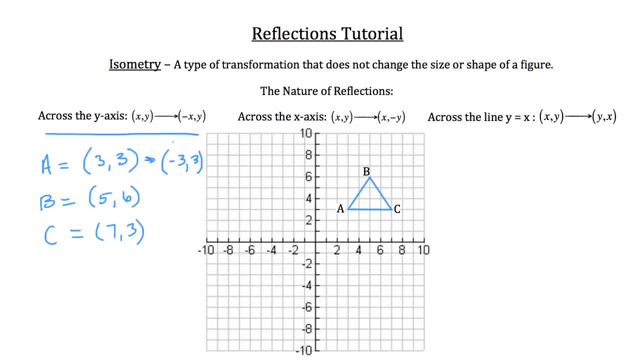 I'm only changing the x coordinate of the point and I'm making it the opposite of what it was. Before it was positive 3, now it's a negative 3.. Same thing for B: It was, now it's. And let's do the same thing for point C. 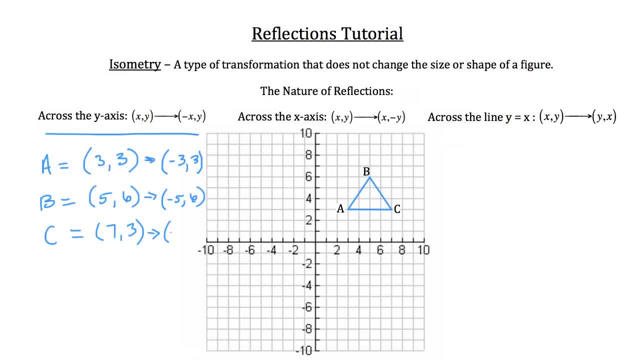 It was, now it's going to be, And I'll go ahead and plot those points on our graph now. The first is A at, So I'll go 3 to the left and then 3 up, and I'll drop a point in. 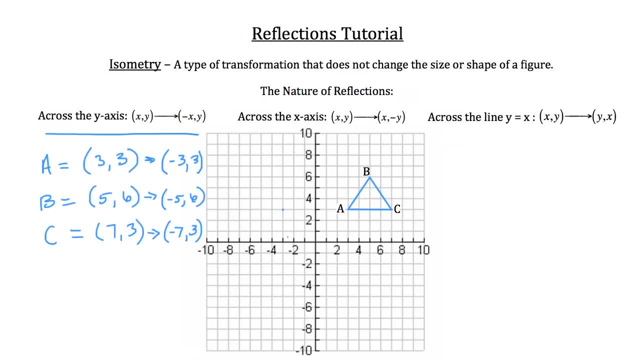 B was at. so I'll go 5 to the left of the origin and 6 up, and we'll drop a point right there as well. And lastly, let's take a look at C It's, so I'll go 7 to the left of the origin. 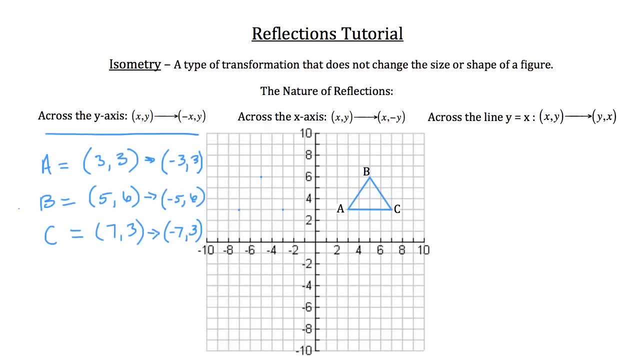 and 3 up, and I'll drop a point. Now that we have those points drawn in, we can go ahead and connect them to form our triangle. Now you'll notice, I've labeled this triangle as A', B' and C' That's what that little apostrophe means. 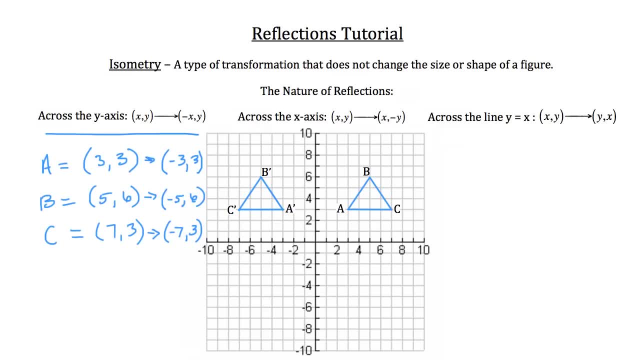 In mathematics or in physics, we call that the prime symbol. So we have A', B' and C' Now that we know how to reflect something across the y-axis, let's move on to the x And notice that we just went directly across the y-axis here. 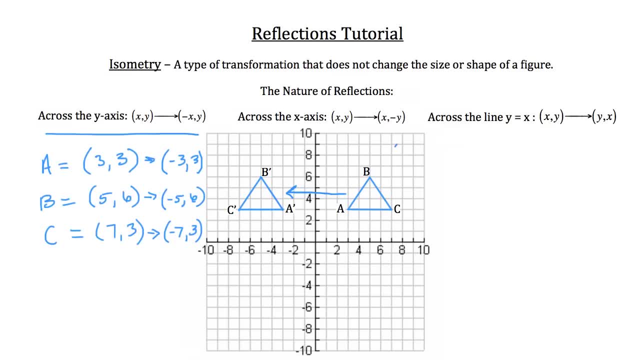 and reflected our image. So this was the original image, called just the image, and this now is our preimage or the isomer of the original image. Alright, so in order to reflect an image across the x-axis, you'll notice that we just have to put a negative. 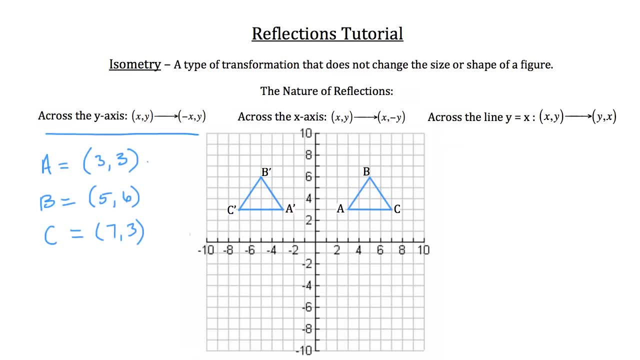 in front of the y-coordinate. So for point A, instead of the reflection is now For B, we had, now we have. And for C: we had and now we have. So now let's plot those three points. 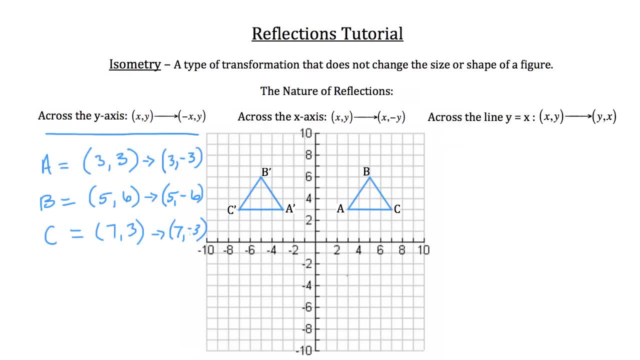 so we're going to go 3 to the right and then 3 down, and we'll plot that point For the new point B we have. so we're going to go 5 to the right and 6 down and drop a point. 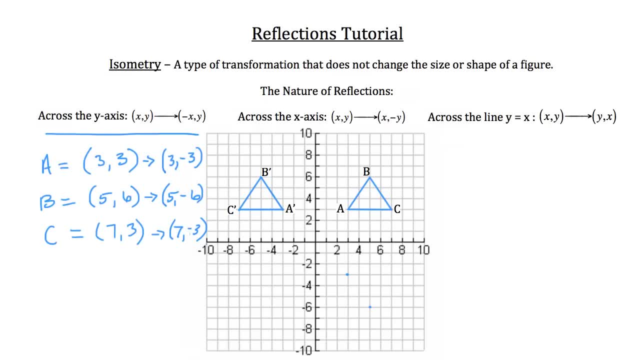 And lastly, for point C, we have, so we'll go 7 to the right and 3 down and we'll drop that point. Now that we have our three points, let's go ahead and connect them and form another triangle. 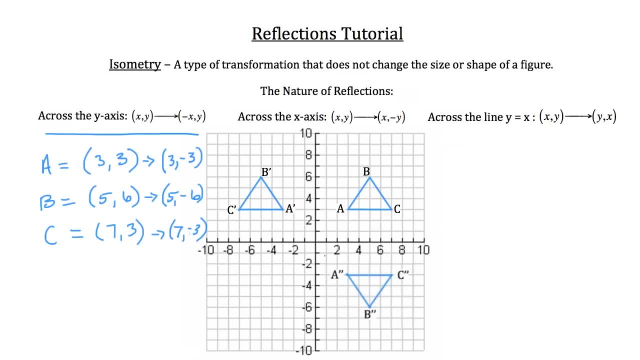 This triangle is double prime because I've already got prime drawn on here. So this is and, And remember, prime and double prime and whatever else you feel like using to label. it is just your system of labeling. what was the original triangle? 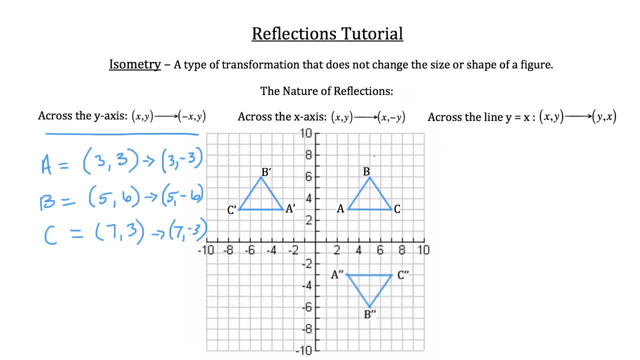 so triangle ABC. And what's your new triangle? It could be prime, it could be double prime. I'll show you an asterisk. It's whatever you want, but prime is really easy. it's just a little, you know, apostrophe. 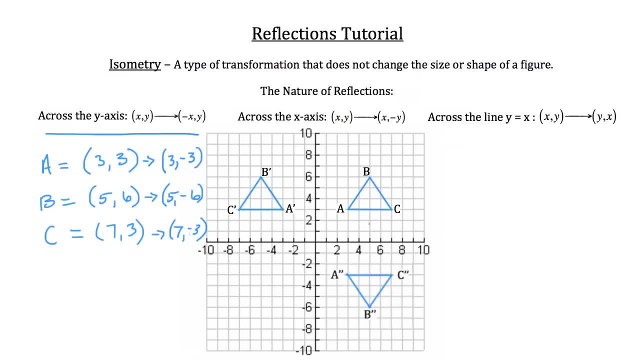 Alright, so this was a reflection across the x-axis and you'll notice we went just straight across the x-axis by making that change and we created our new triangle, Double prime triangle, ABC. So, lastly, let's go ahead and reflect. 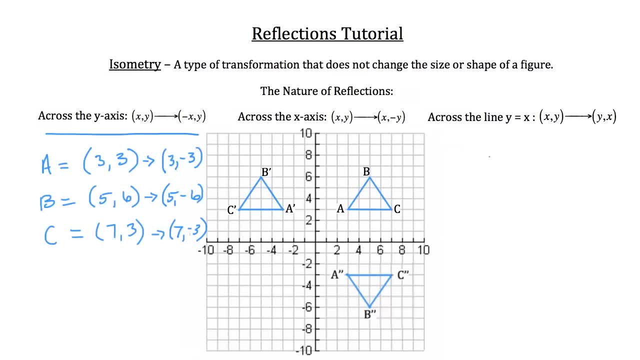 that original triangle, triangle ABC across the line y equals x. And remember, if you were to draw that line y is equal to x, it would look like this, Like this red line here, it's just a line cutting through the origin. 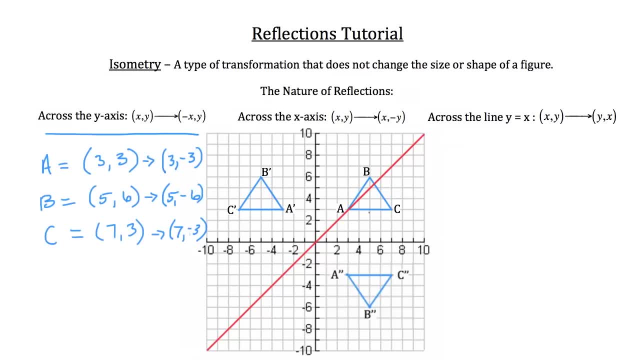 with a slope of one. So now we're going to reflect triangle ABC across this line. In order to do that, we want to take our original xy coordinate and change it to So for a it was originally. we're just going to switch the x and y. 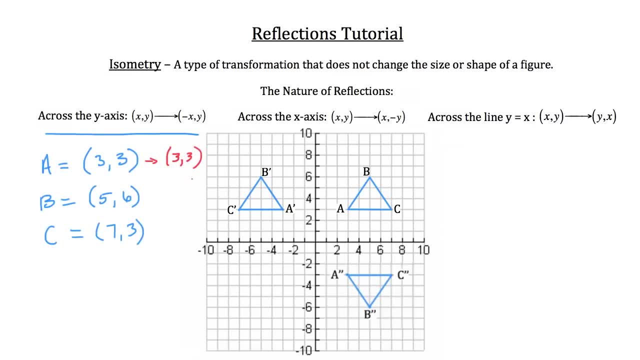 and it's going to remain. as b was, so now, reflecting across the line, y is equal to x, it becomes. And lastly, c was so, that becomes So. now we just want to plot those points. Our first one, a, is. 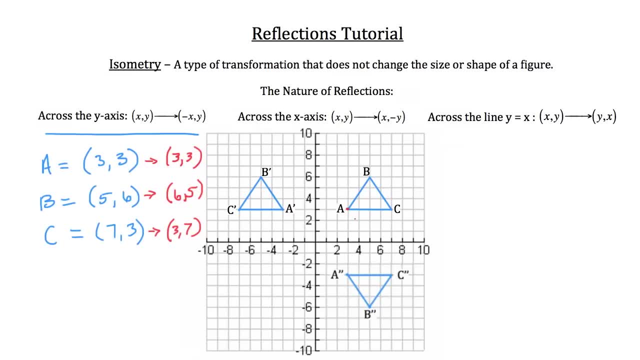 It hasn't changed position so I'm going to just drop it in right there. b is so we can go 6 over and 5 up and drop a point right there, And c is so we go 3 to the right of the origin.